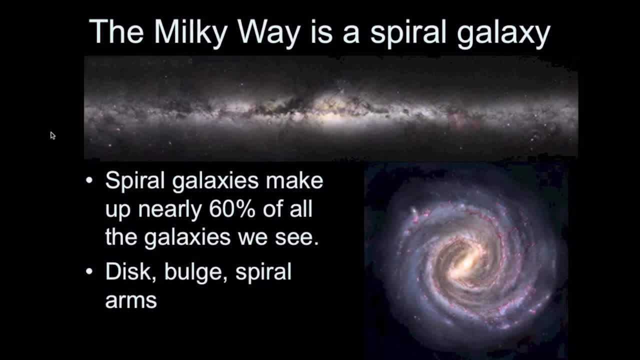 shows our view from inside of the galaxy. The sun is in the disk of the galaxy, and so when we look through it, we see gas and dust- that's the dark material that we see within the disk, and then we also see the light from stars within the disk of the galaxy. 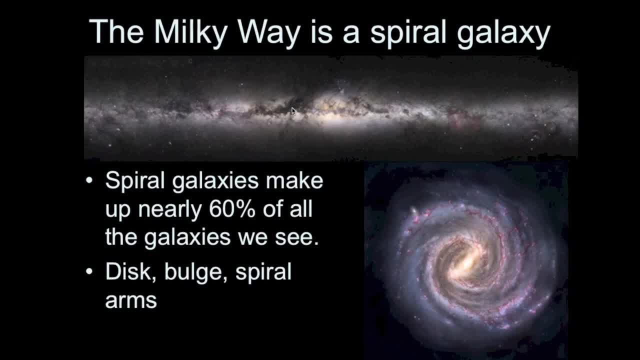 And then we also see the light from stars within the disk of the galaxy, And the image on the bottom right is what our galaxy would look like if we could see it top down. So spiral galaxies make up about 60% of the galaxies in our local universe. 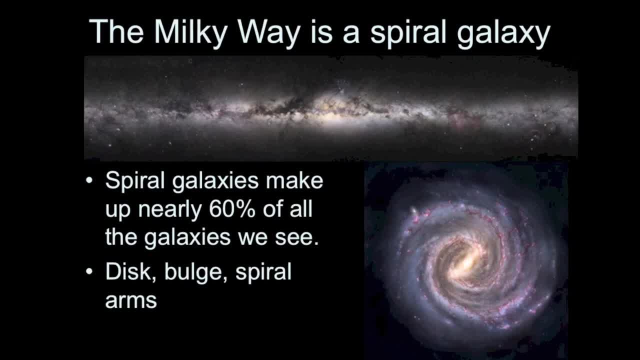 the ones that are easily seen through a telescope, And spiral galaxies are generally made up of a disk of stars, gas and dust, a bulge near the center and spiral arms. There's a few different types of shapes of spiral galaxies. 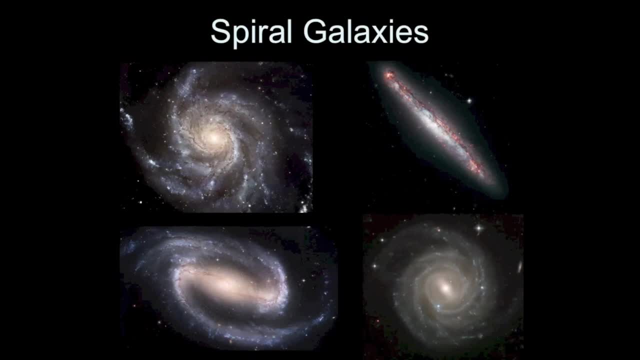 I've got a few here, seen top down and edge on A spiral galaxy like the one in the top left. here we have some very nice spiral arms, gas and dust. On the bottom we see a spiral galaxy with two big arms, a bulge and a bar through the center. So there's something. 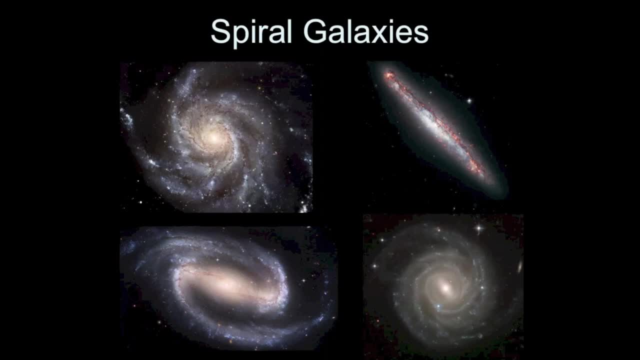 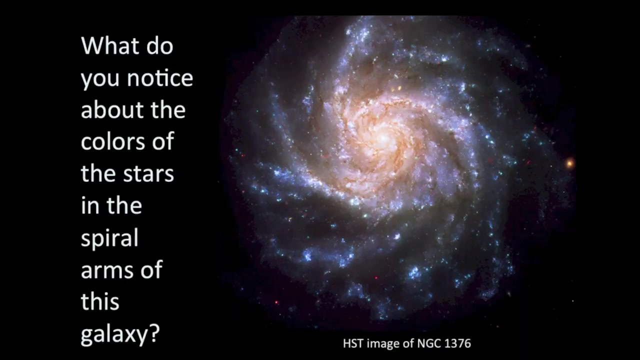 also called barred spiral galaxies. On the bottom right is a barred spiral galaxy, but also with a ring around the bar, And then in the top right is a spiral galaxy seen edge-on. Let's take a look at this image of a spiral galaxy. 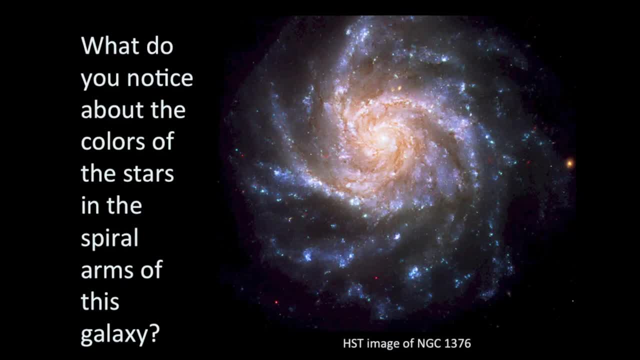 This is NGC 1376, and this image was produced by collecting light with the Hubble Space Telescope. Let me ask you this question: What do you notice about the colors of the stars in the spiral arms of this galaxy? If you thought that what you mainly see is blue color, then you'd be right. 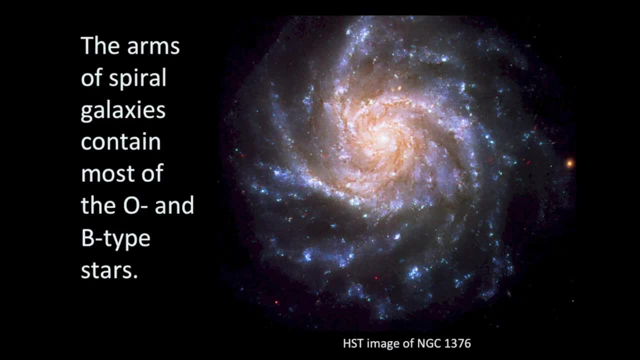 And blue stars are mainly O and B-type stars. What this means is that the arms of spiral galaxies contain most of the O and the B-type stars, because it's not just this galaxy we notice this with. We notice this with most big spiral galaxies. 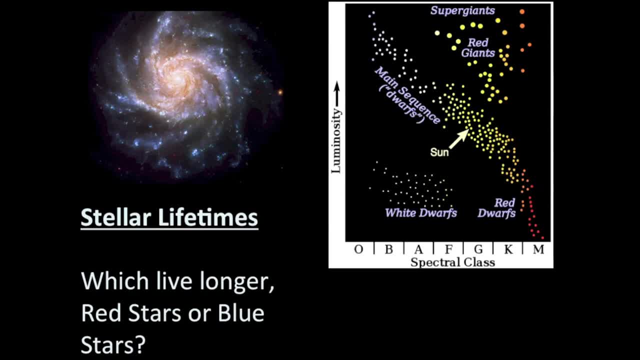 So here's another question: Which stars live longer, red stars or blue stars? If we're talking about blue stars, we're probably talking about the O and the B main sequence stars, And with red stars I'm not really talking about the red giants. 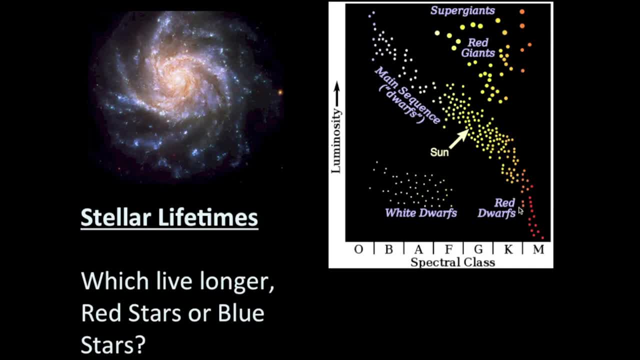 I mean red main sequence stars, And so the ones that live the longest are the ones that are the lowest in mass And, as we've discussed before for main sequence stars, the lowest mass ones are the ones with the lowest luminosity and the lowest temperatures. 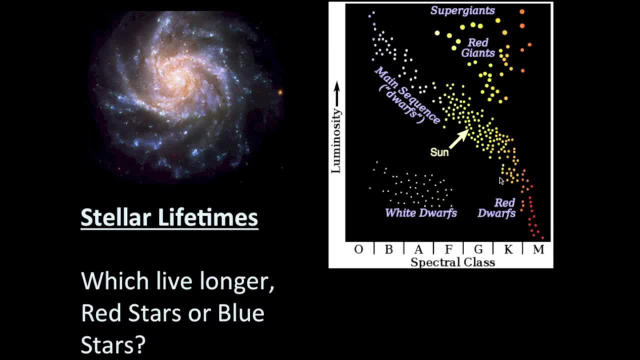 or the redder main sequence stars. So the red stars live the longest, which is the ones that live the longest, Which means blue stars live a shorter amount of time. So what we can conclude from this is that stars in the spiral arms of galaxies 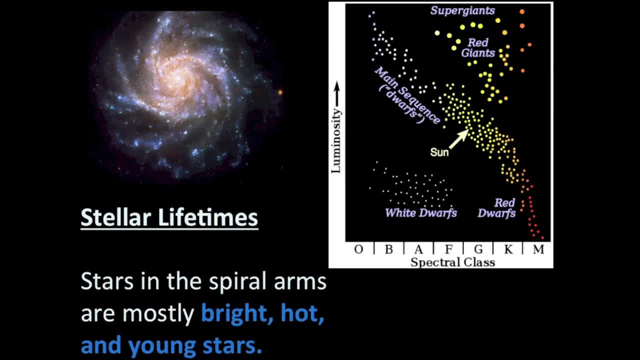 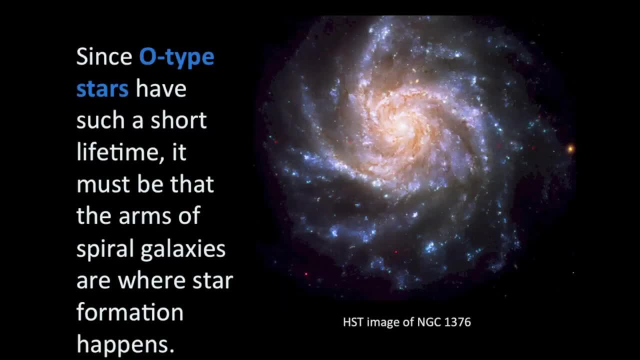 are mostly hot, bright and young stars. There's stars in between the spiral arms, but they're not primarily the O and the B-type stars, And since O-type stars have such short lifetimes, what this means is that the spiral arms 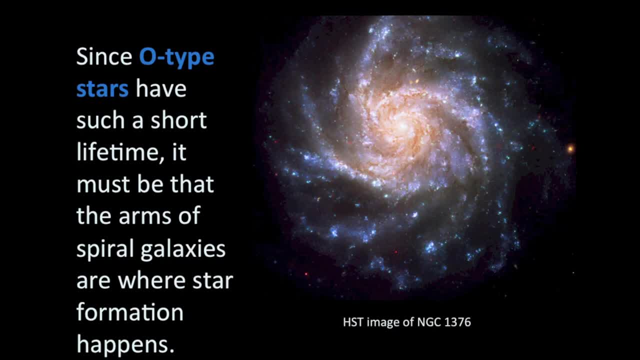 is where stars form. Because the O and B-type stars? because they don't live very long if they're in the spiral arms. they haven't been there for very long and they haven't had enough time since forming to drift out of the spiral arms. 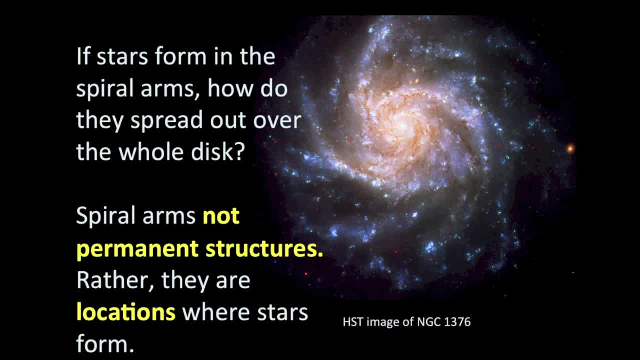 So if stars form in the spiral arms, how do they spread out over the entire disk of a spiral galaxy? We have to remember that spiral arms are not permanent structures. Rather, they're just locations where stars form, And stars can drift from a spiral arm into another part of the galaxy. 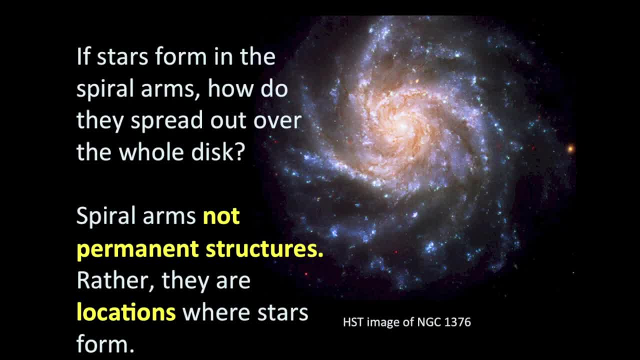 over the course of its orbit, But if it's an O or B-type star, it's not going to have enough time to do that. It will be seen only in the spiral arms because it will be born. it will live for just a few million years. 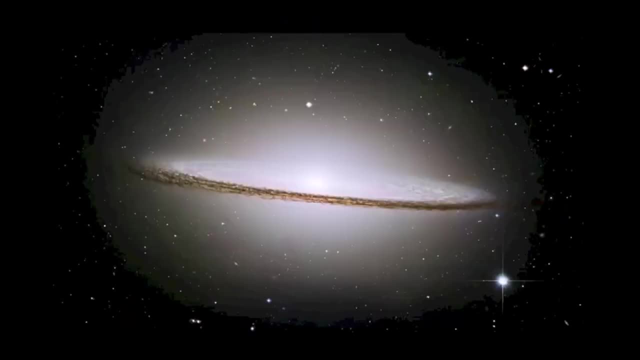 and then blow itself up. I have some images of other galaxies to show you. This is the CIMBRA. This is the CIMBRA, This is the CIMBRAO galaxy, and what we're seeing is a lot of bright emission from stars. 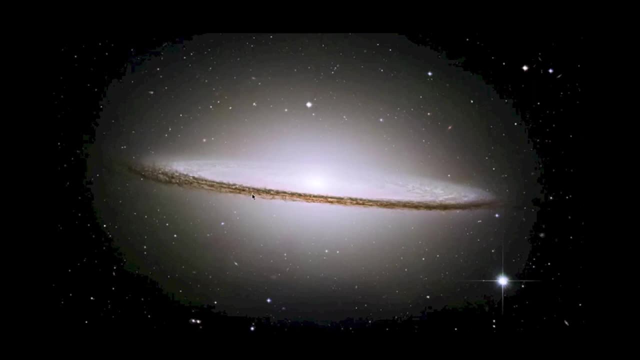 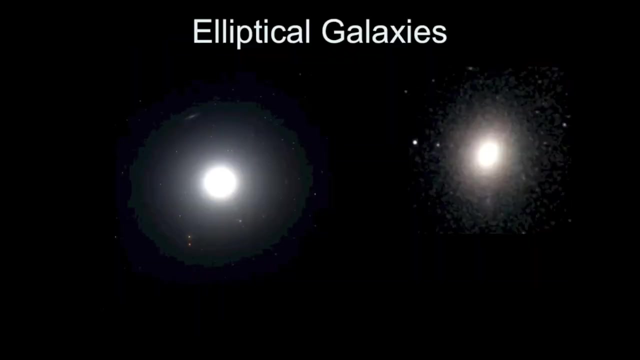 and then we also see a dusty lane or a ring in a disk around the large bulge of this galaxy. There's other galaxies that don't have a disk appearance, and these are called elliptical galaxies. They can be very round in shape. 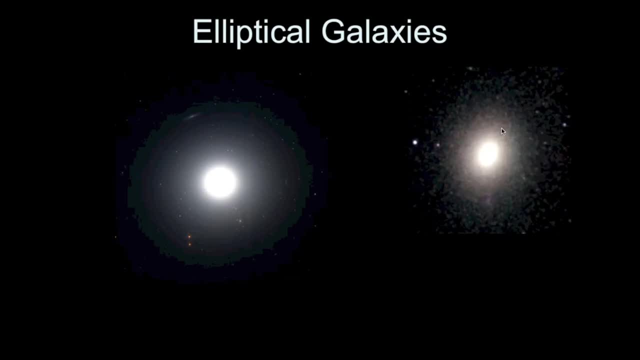 or they can be kind of football or egg-shaped. And the elliptical galaxies have an other peculiar feature about them, Or rather they're missing a feature that the disk galaxies have. What we don't see in elliptical galaxies is a lot of blue stars. 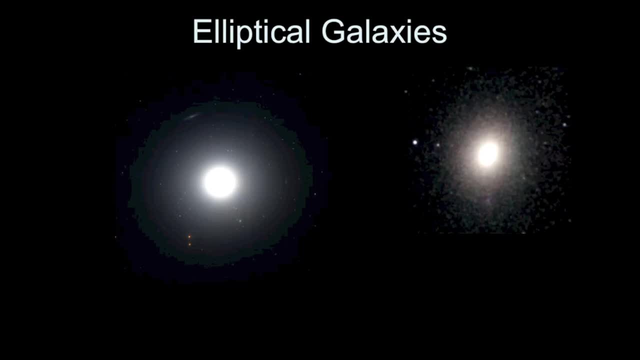 and we also don't see a lot of gas and dust, And what that means is that the elliptical galaxies probably have a lot of old red stars in them. Does this mean that there were never any blue stars in an elliptical galaxy? Well, no, but it could be that the blue stars were there in the past. 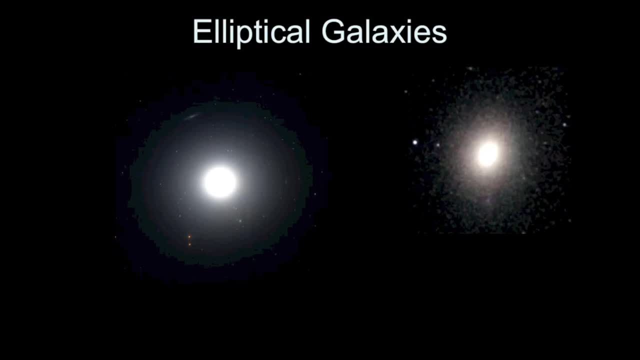 but they're just not there anymore. And where did all the dust and gas go? We're not exactly sure, But what we do know is that elliptical galaxies probably don't have a lot of star formation, because star formation needs dust and gas in order for that to occur. 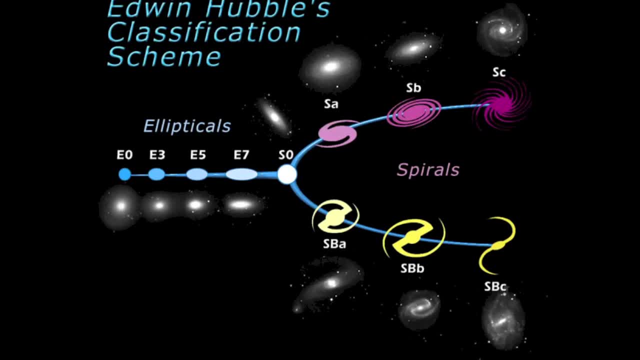 In the early 20th century the American astronomer Edwin Hubble came up with a classification system for galaxies- And today astronomers call it the tuning fork, and Hubble's classification scheme went from the rounder ellipticals being called E0,. 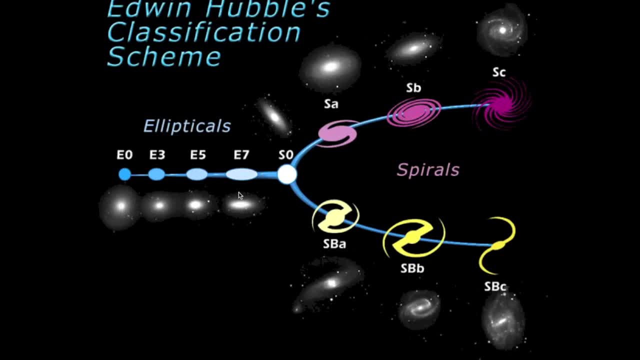 and as you go up to a higher E number you have a more squashed appearance. for ellipticals, then lenticular or galaxies that have kind of a weak division between elliptical and spiral would be maybe an S0. For spiral galaxies: 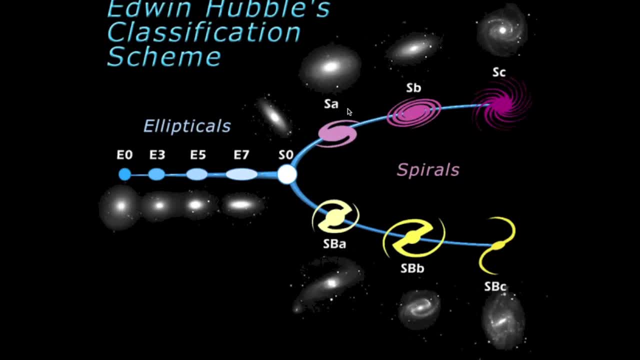 that don't have a bar through the center. Hubble classified them as SA, SB and SC. SA had perhaps fewer spiral arms that were less tightly wound And as you go to barred spiral galaxies you'd have SBA, SBB and SBC.